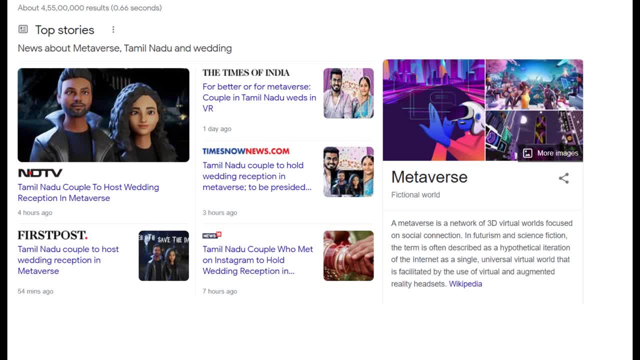 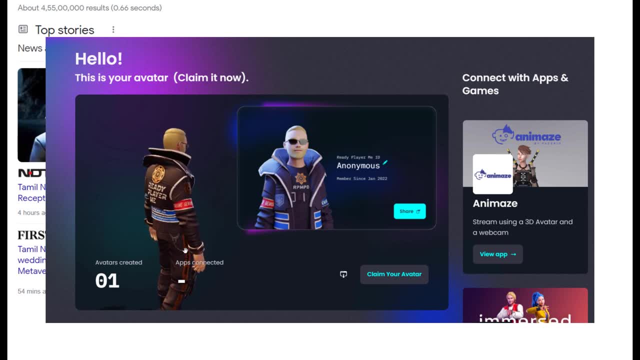 like in the form of an avatar. Not like the avatar, a blue-tailed avatar that you see in the avatar movie, But your 3D holograms, so called avatars, will see or live in the virtual world. In this virtual world, you will meet everyone from your home directly. They could be your members, family. 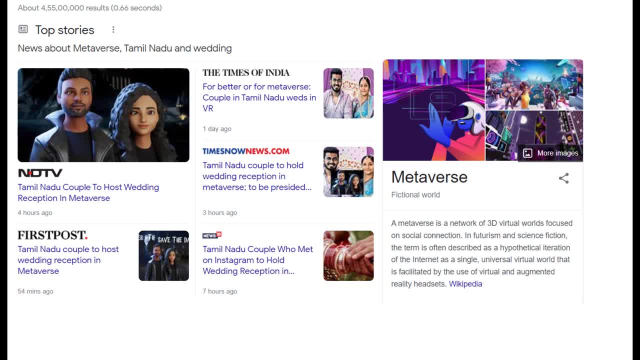 members, friends, or there could be a strangers as well. Like you meet on Facebook, Facebook, you can meet strangers on Facebook, add as a friend and so on. The tomorrow is very near- not so far- and tomorrow's metaverse has pros and cons. If you have habit of watching news, 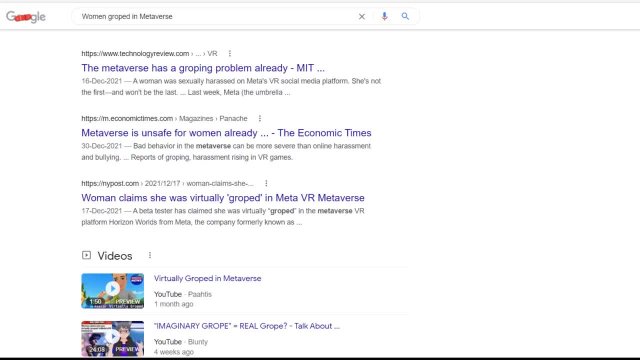 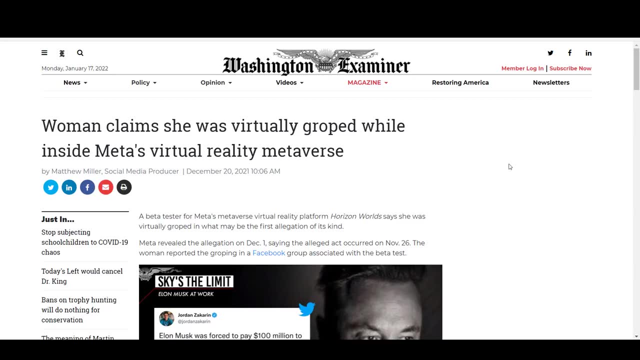 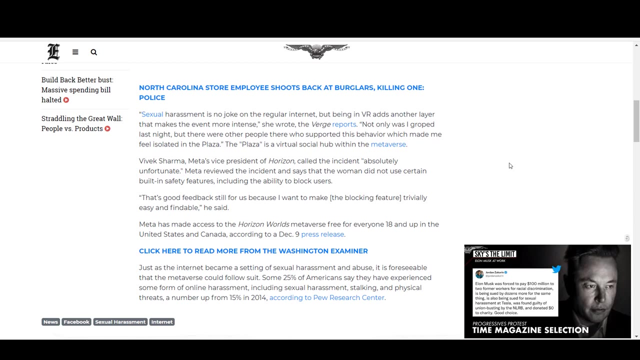 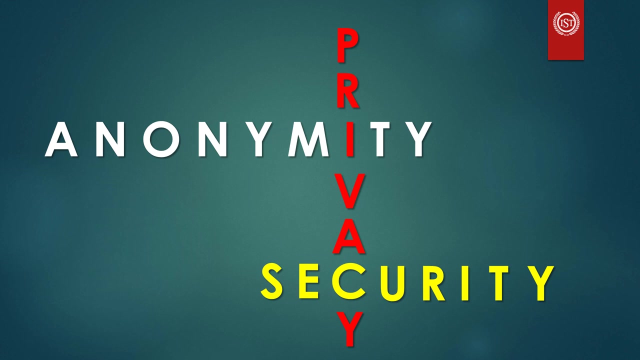 you must have heard the news that woman was grouped in metaverse virtual reality platform. that's horizon, and that was a sexual harassment and it is a serious concern that needs to be addressed. And if teens and kids are exposed to embarrassing events like you, know what to say. it's hard for me to say that a new type of porn is already. 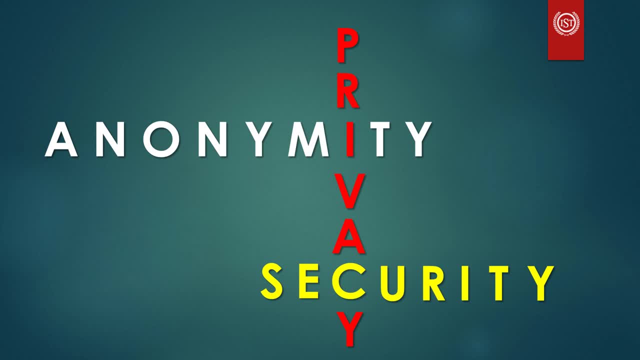 set to exploit virtual reality platforms and if your family members, whether teens or kids, encounter that, that embarrassing- what to say, that embarrassing avatars, that could be really worse. that could affect the mentality of the kids and teens And, as you can see, this. 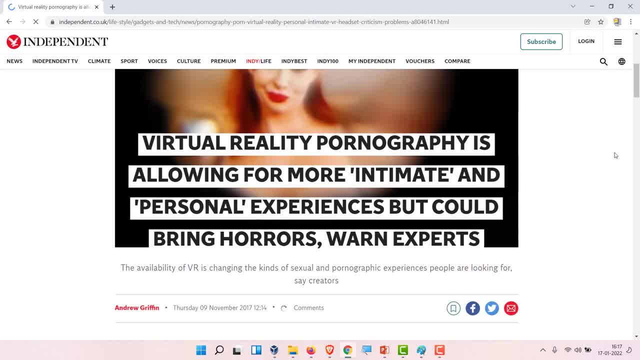 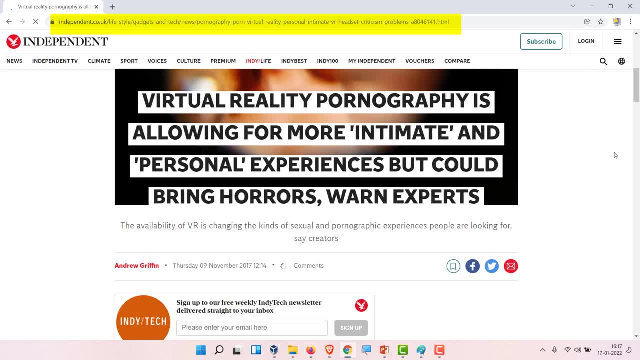 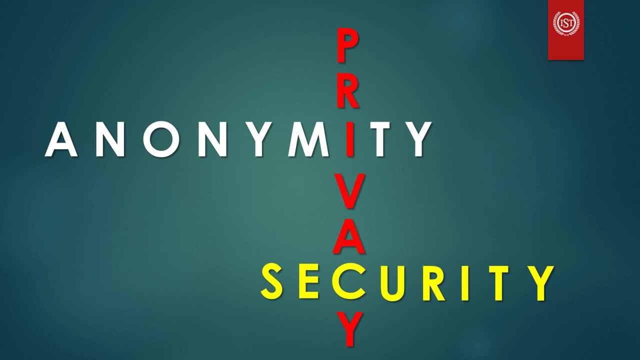 article. virtual reality pornography is allowing for more intimate and personal experiences, but could bring horrors Once experts. you can see or read this article in this link. So everyone, not only you, but your friends who are non techies, like doctors, engineers, teachers. 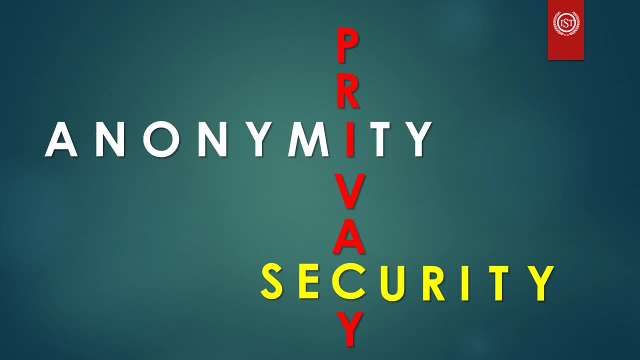 other workers. businessmen should know the importance of being secured. That is security practice, privacy and, if necessary, must stay anonymous if required. As you know, if you are getting something for free, then you are the product. This is a famous saying. let me repeat: if you are getting something for free, then you are the. 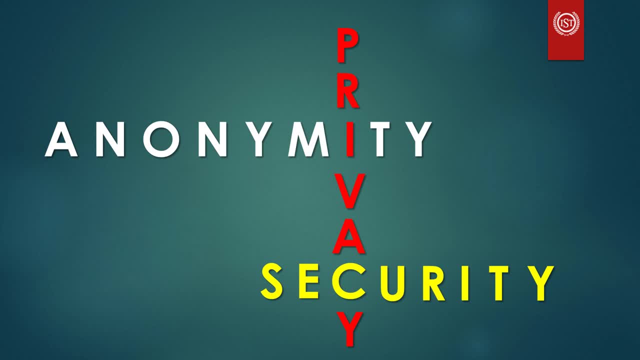 product, So you may say that you have nothing to hide. but you are the product, So you should hide, You should practice of being anonymous. But it is also true that when you keep high security or when you practice high security or privacy, You will have a least comforts. 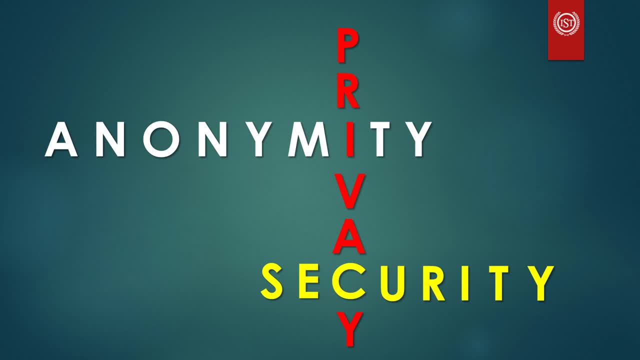 or less comforts В één сейф, отсутствие colors. В один мая у меня естьcession, soaking из-за لمнали солнце когда я tweeted signboards. apart from metaverse on the internet, you are daily invaded, right? your privacy is invaded daily and 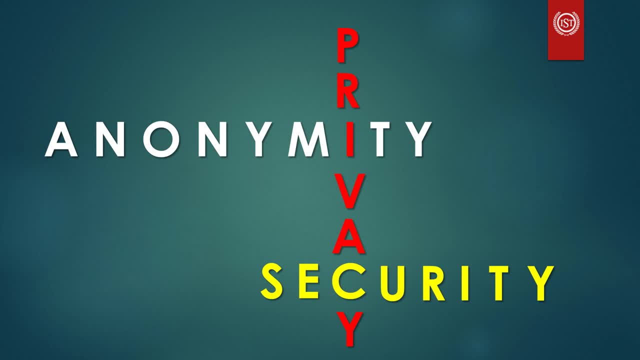 you don't even realize that what harm is causing to you. they hope you understand or you can assume to whom i refer, as they they keep tracking all your activity daily, every minute. they place cookies on your systems devices on the name of better experience for customers, but the motive is more. 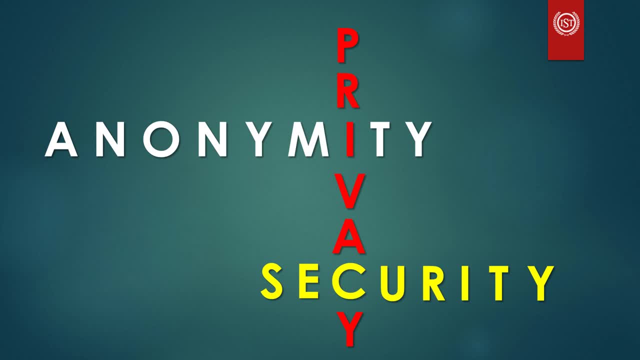 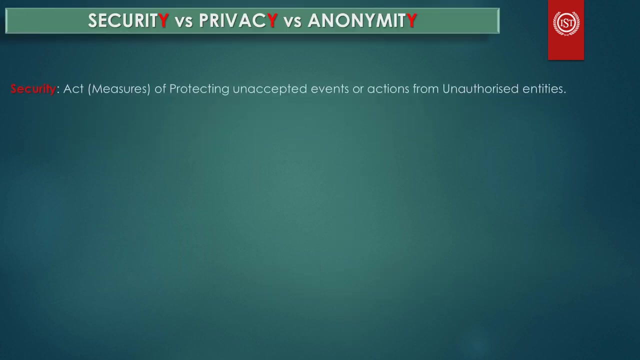 than bad, worst intentions they have. they are playing with your psychology. it's a mind manipulation techniques. so you must have privacy. if possible, try to hide yourself. so what is security? privacy and anonymity. you already know what is security. you have learned this terminology in the first module of this course. security is an action or measures to take or to protect yourself yourself. 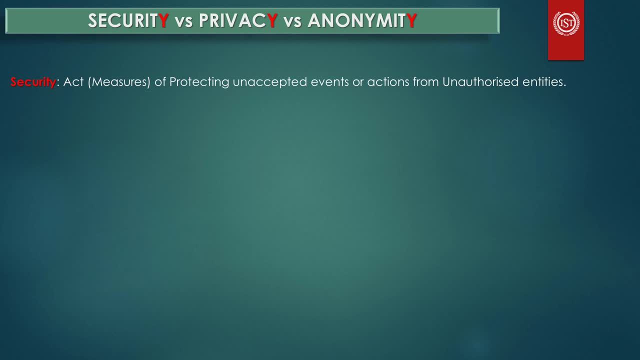 means physically, you or your devices. physically and digitally, your activity. So protecting your activity from unauthorized persons, institutions and applications, and so on. Installing antivirus applications can protect your computers to some extent, but they are not 100% effective. So now, what is privacy? 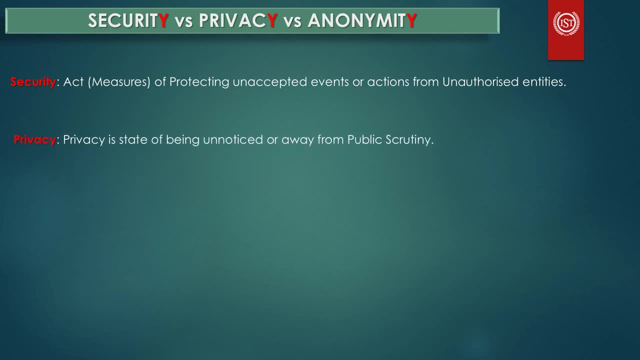 Privacy is state of being free from public notice or public observations or public scrutiny, Or you can say freedom from intrusions or interferences from something or some persons. For example, if you are in your home with your family, having lunch together, playing with your kids or having happy time with your spouse, husband or wife. 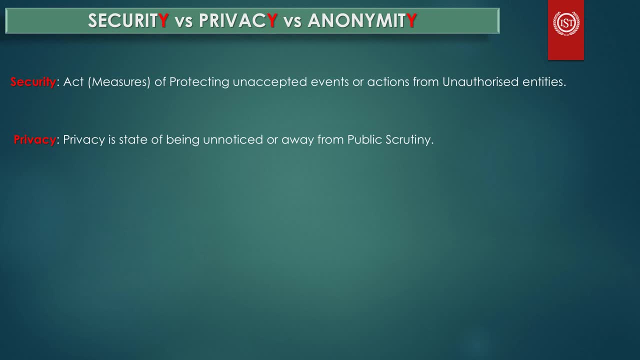 People outside your house- neighbors- knows that you are inside, but they don't know your activities. This is an example of privacy. Guys, I know what I am telling to you. Most of the men and women on internet they are using, or you might be using, incontico, google incontico tab for privacy on internet. 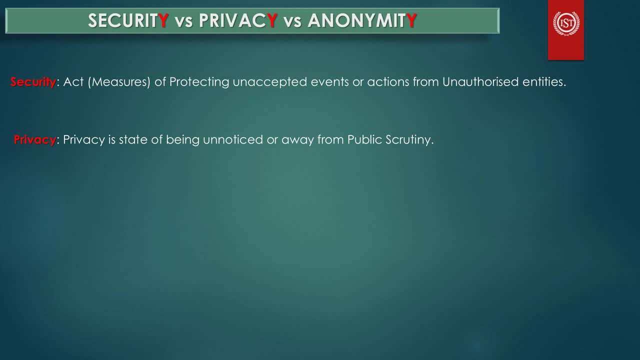 I know what kind of webpages, I know what kind of websites you or they might be visiting. That's not a privacy. Your ISP knows what activity is running on your system or what network traffic is coming and going from your computers or devices. 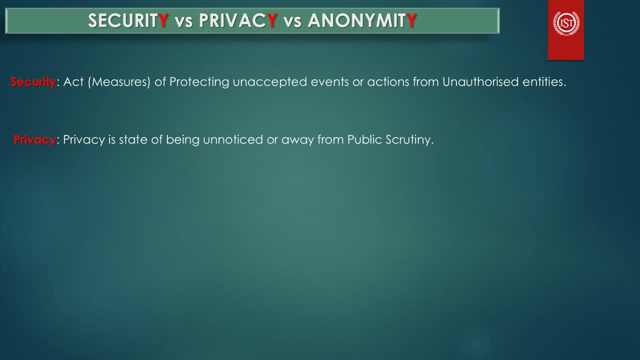 Like phones or tablets, Google, incontico or any other browser which is providing privacy is not exactly privacy. It only erases history, browser history and browser caches. That's it. Your ISP knows and logs your activity. If required, your ISP knows and logs your activity. 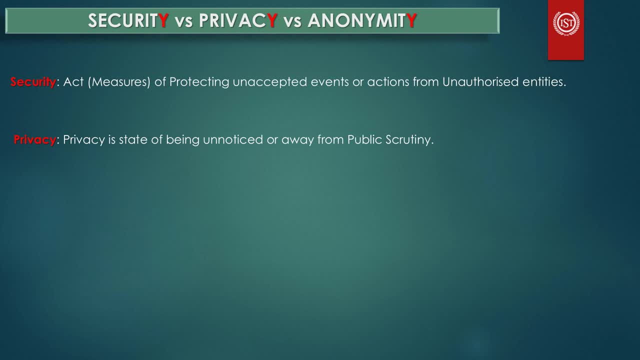 If required, your ISP knows and logs your activity. Your ISP submits your log activity to law enforcement department if necessary, if it was a cybercrime cases, and so on. So educate yourself and teach to your well-wishers. It is very much important. 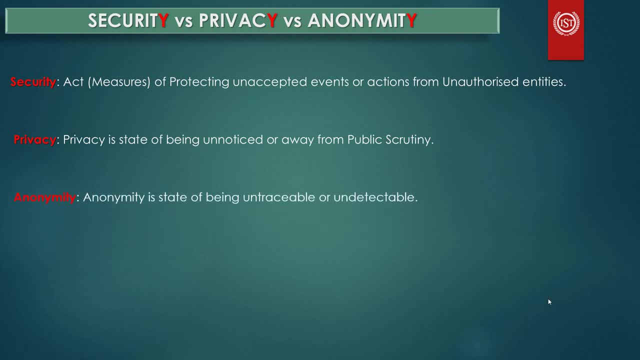 And next, what is anonymity? Anonymity is actually an ability to make yourself undetectable or untraceable or untrackable and so on. Your activity can be logged or identified, But the source of your activity or you is literally untraceable or untrackable. so that's what anonymity is. the example of anonymity is: 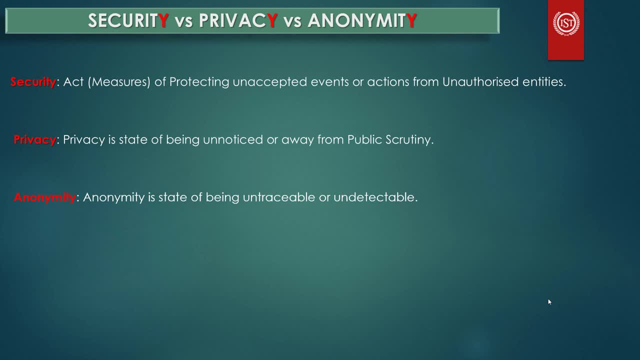 whistleblowers. i hope you know who is a whistleblower is. if you don't know, whistleblower is a person who exposes any illegal activity, harmful activity or crime that is done by persons, institutions or organizations and reveals it to a general public using any media or a platform. so that is a whistleblower is. and whistleblowers prefers to stay anonymous. 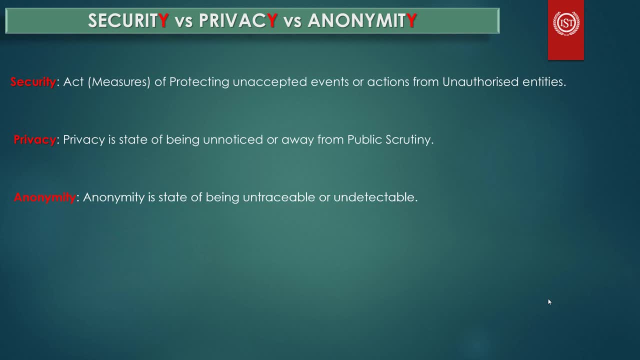 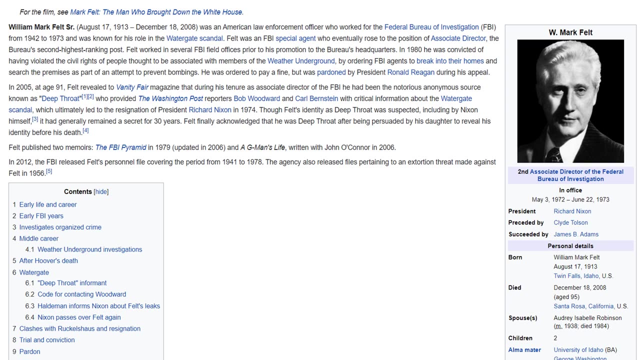 and reveals important information to the public. the best example is mr mark felt. if you have a habit of reading news, you must have known who is mr mark felt is. mark felt is law enforcement officer and worked in fbi and he exposed so many scams and scandals, one of which famous scandal is. 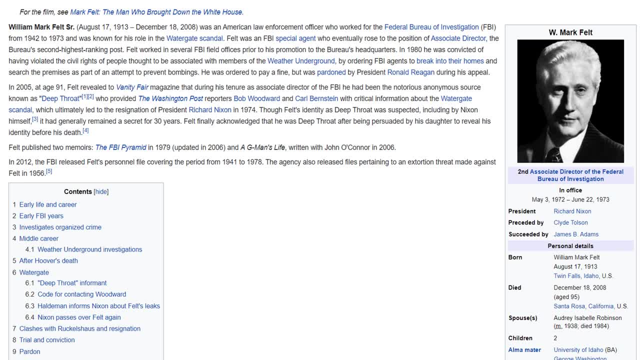 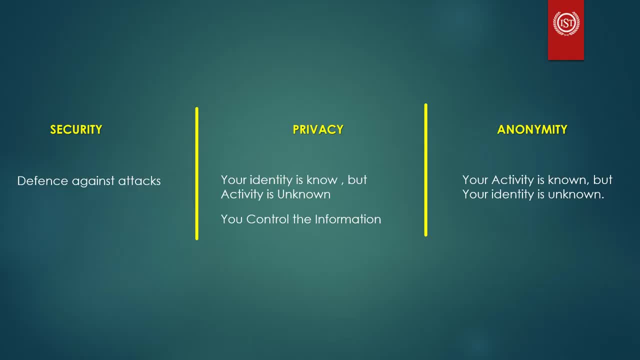 fbi wargate scandal. you can search on the internet and he was anonymous for decades while exposing these scandals. so that is what anonymity is. so, as you can see on the screen, i said there is a hairline difference between these three terminologies. security is defense against attacks. 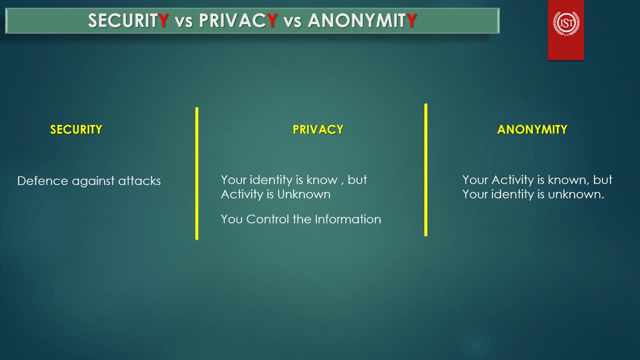 privacy is where your identity is known, but activity is unknown. in here you actually control your information. while anonymity is, the activity is known, but the source or identity is unknown or untraceable. so, dear friends, your personal data is a dangerous weapon that you are giving yourself.